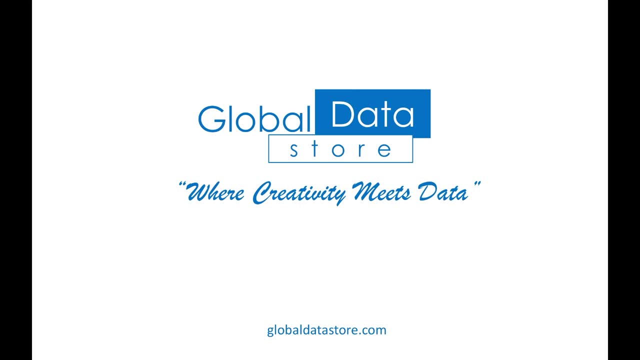 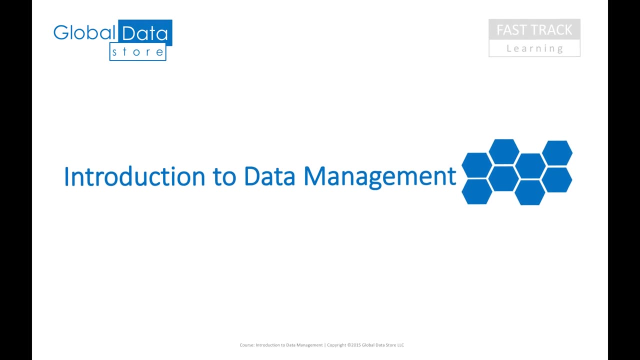 Welcome to Global Datastore, the place where creativity meets data. We are glad to have you on Introduction to Data Management course, which is our signature course. If you are looking to learn the key aspects of data management, you are on the right place. 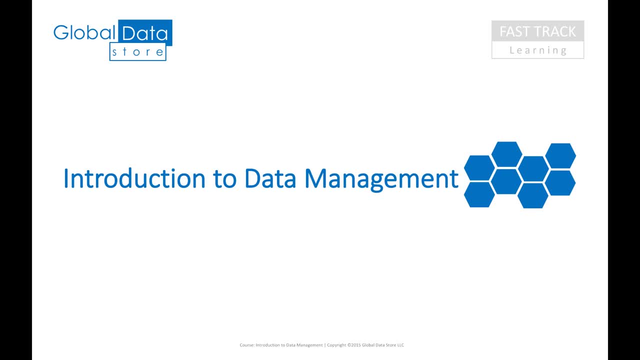 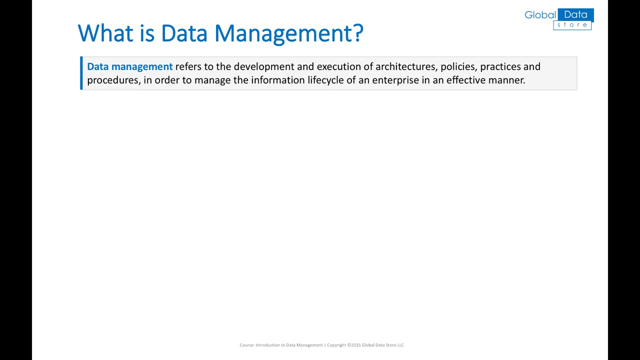 By using fast-track learning method designed by our experts. we hope you will enjoy an exceptional and time-effective learning experience. Ready to start, Let's go to brief course overview. This course is about data management, So let's define what is the data management. 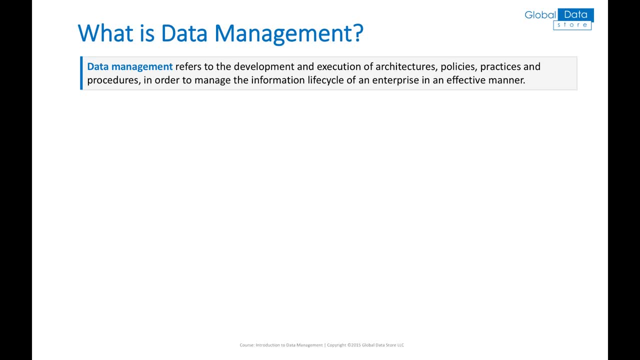 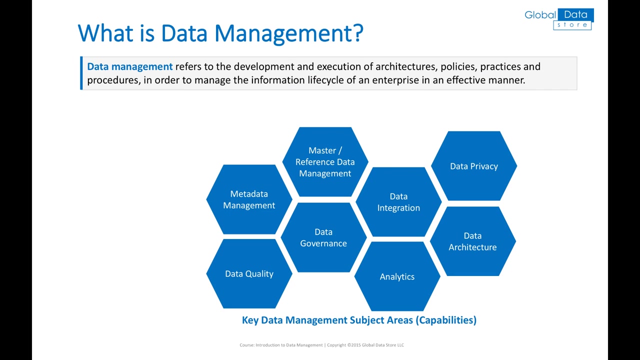 Data management refers to development and execution of architectures, policies, practices and procedures in order to manage the information life-cycle of an enterprise in an effective manner. The key data management subject areas are metadata management, data quality, data governance, master and reference data management, data integration, analytics, data privacy and data architecture. 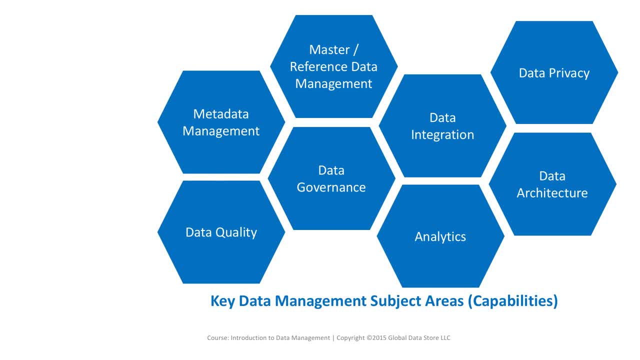 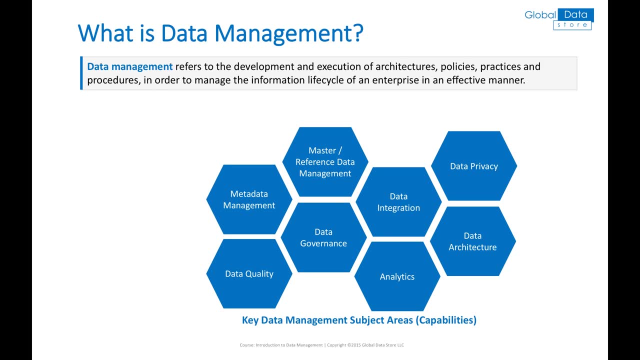 Data management subject areas are also called capabilities. Each capability has three aspects: People refers to organizational aspect. the roles and responsibilities required for the capability. Process refers to activities that are associated with the capability. And three: technology refers to technologies and tools required to support capability: business processes. 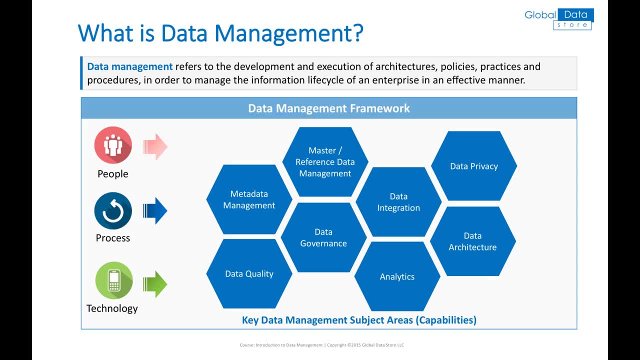 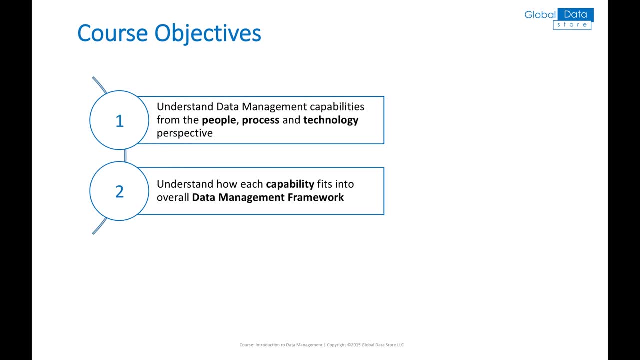 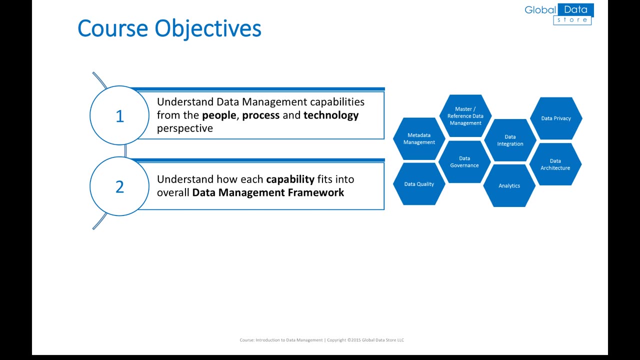 Data management subject areas are closely related and have synergized influence to overall data management framework. Now let's define the course objectives. In this course we are looking to: 1. Understand data management capabilities from the people, process and technology perspective And 2. Understand how each capability fits into overall data management framework.